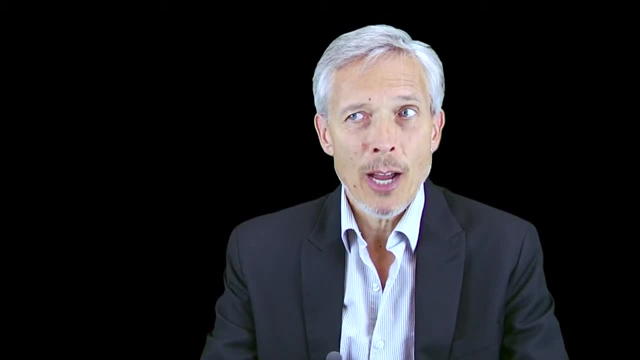 the curtain raising of the universe when it became transparent for the first time. Its temperature when this radiation was emitted was about 3,000 degrees Kelvin, And the universe has expanded a thousand fold since then, stretching the radiation from the universe to the atmosphere. 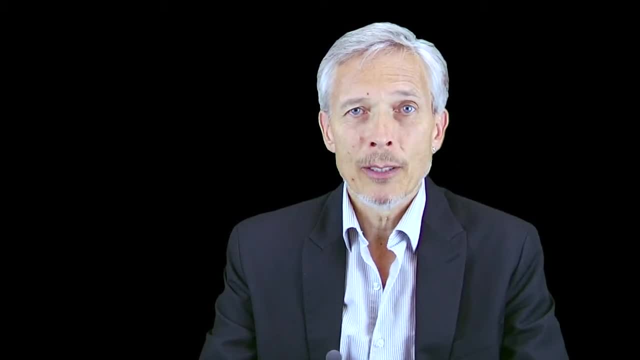 So this radiation represents a baby picture of the infant universe in its very early hot phases. The microwave background radiation by a factor of a thousand in wavelength to become microwaves. Because the microwave background radiation, as it's called, is such a signature of the 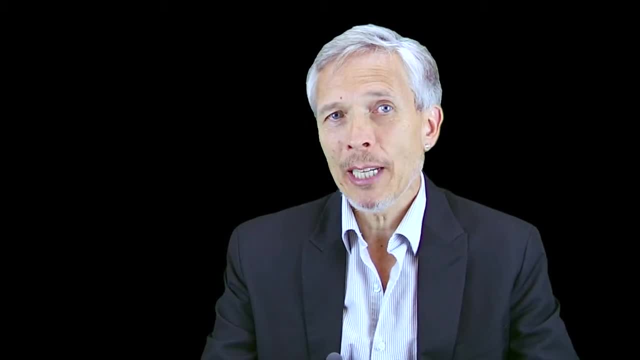 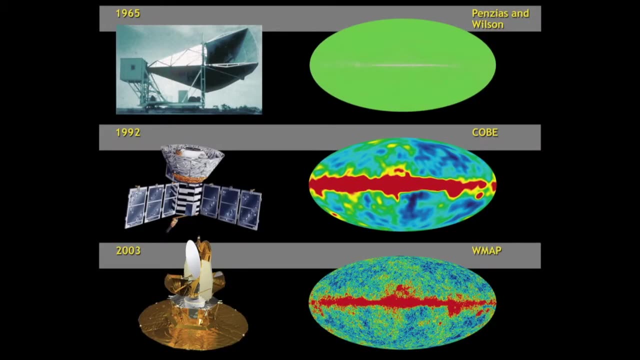 Big Bang. enormous effort has been put into measuring it more precisely and understanding it in detail. The first map of the sky produced by Penzias and Wilson showed a uniform signal of microwaves at a temperature just below 3 degrees Kelvin, almost absolutely cold. 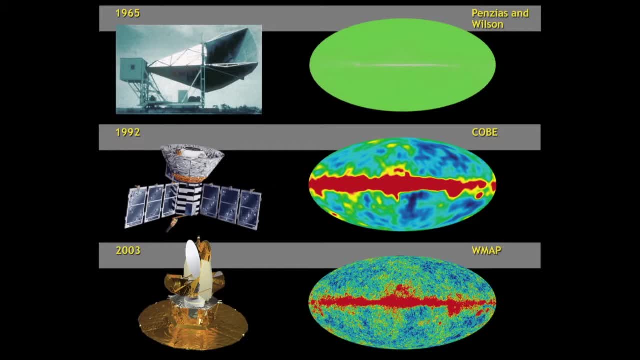 Astronomers were motivated to learn more about the microwave background. In the late 1990s, NASA launched a satellite called the Cosmic Background Explorer. COBE COBE produced a map of the microwaves that started to show detail. The central region of the map represents 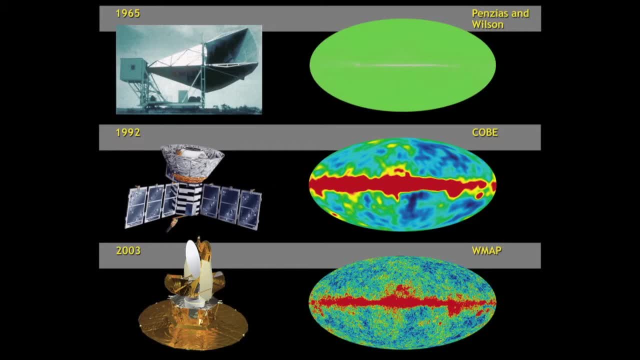 emission from the Milky Way. so that's a proximate signal that gets subtracted out to analyze the universe as a whole. COBE data showed the hints of fluctuations in the microwaves that were assumed to be the seeds for galaxy formation. In breathless press releases of 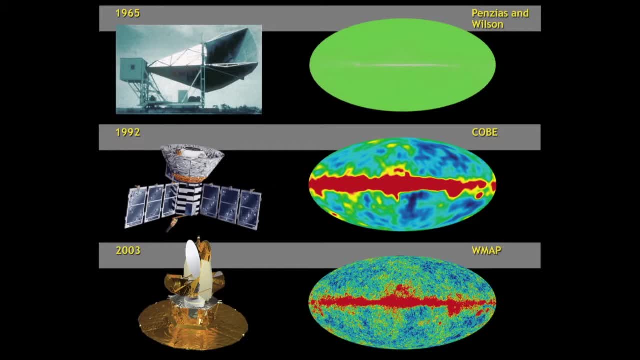 the time, people talked about discovering the fingerprints of God, But COBE barely showed or hinted at these fluctuations. so designs were made for a new satellite, WMAP, the Wilkinson Microwave Anisotropy Probe that would explore this radiation with 10 or 20 times better. 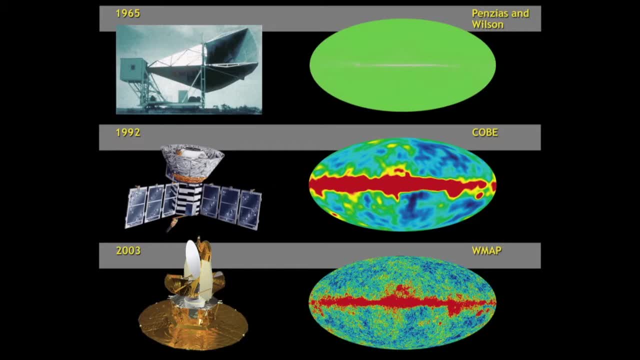 signal-to-noise in resolution. WMAP operated for most of the first decade of the 21st century and produced exquisite detail of the microwave radiation, refining and honing our theory of the Big Bang. One thing these microwave satellites are able to do, especially WMAP, is explore the nature. 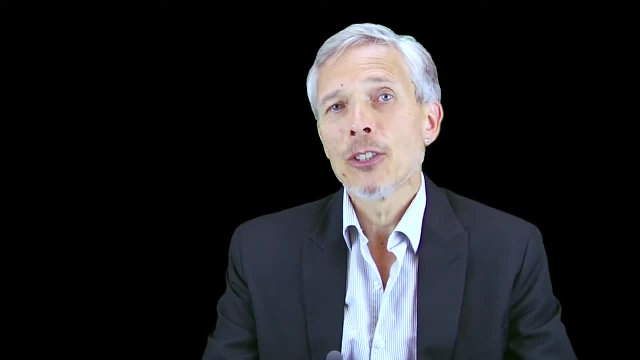 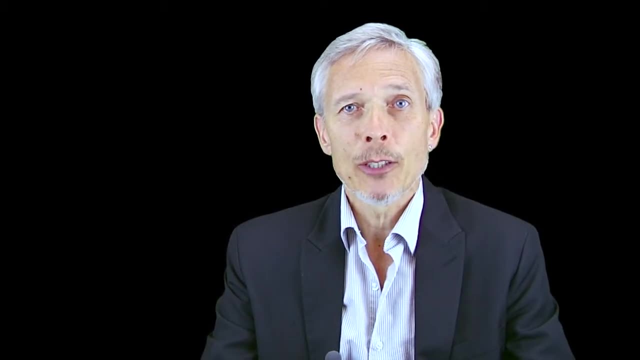 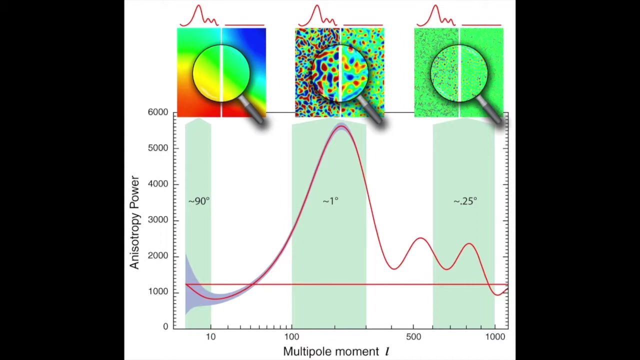 of the angular fluctuations of the microwave. Now that we know the radiation is not completely isotropic or uniform, we can look at on what spatial scales or angular scales the radiation fluctuates. If you look at the WMAP picture, it has the illusion of speckling on a particular scale, And that's not an illusion, mathematics. 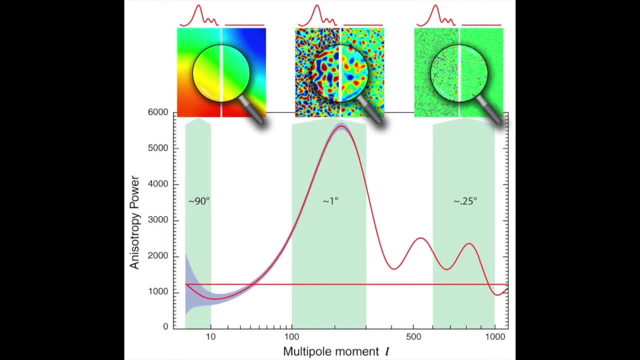 shows that there is a preferred angular scale for the variations In these maps. color is coding temperature, but those differences are tiny, less than thousandths of a degree kelvin. The angular fluctuation power spectrum or the angular fluctuation power spectrum is: 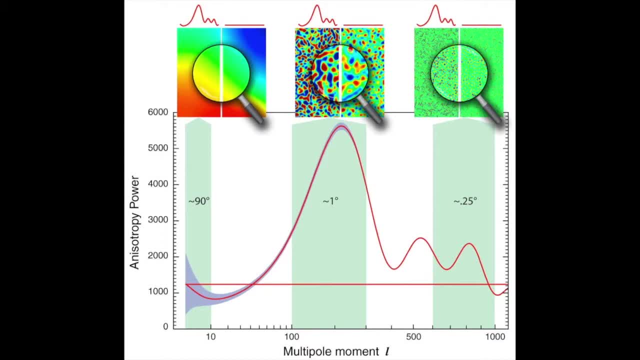 the amount of power in the microwaves on different angular scales shows a peak at about one degree. This is a characteristic of the physics of the very early universe and needs to be explained by the Big Bang model. There also is a second and a third peak at even smaller scales, and 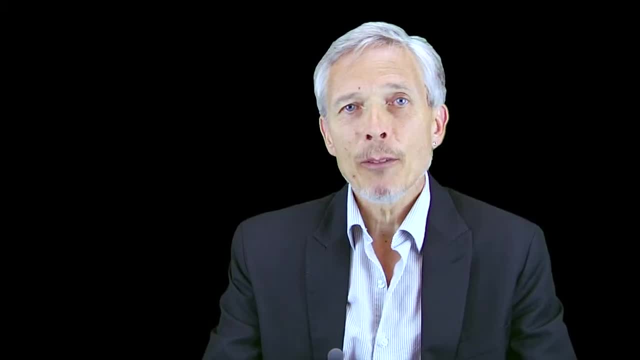 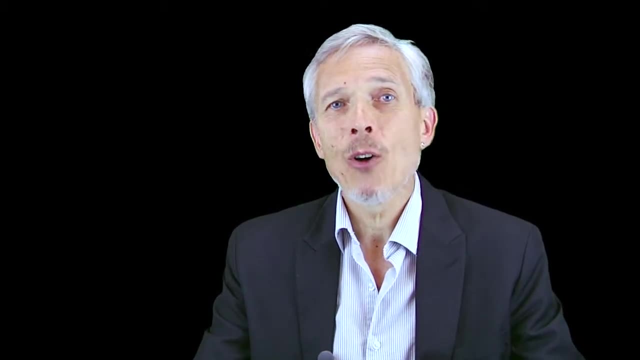 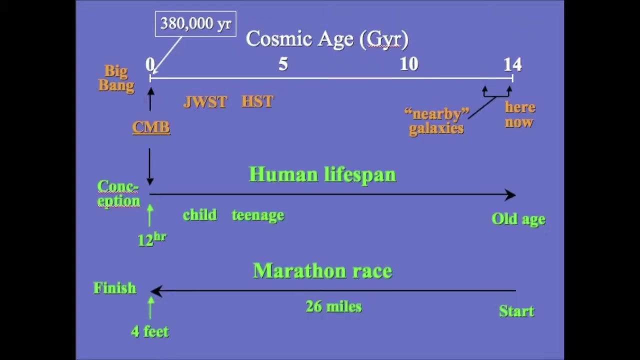 this is also helping us understand the Big Bang better. This level of detail is unprecedented and came only with the WMAP mission. We can use a timeline analogy to realize how early a picture of the universe these microwave observations are giving us. The universe is 13.7 billion years old and the microwaves have helped tell us this age. 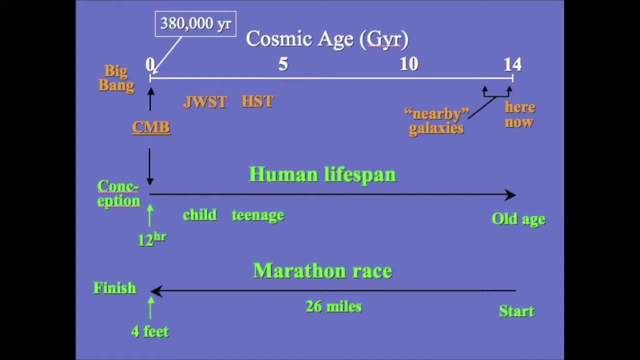 with precise detail, perhaps an accuracy of three or four percent, But the microwaves were imprinted 380,000 years after the Big Bang, As a fraction of nearly 14 billion years. this is a tiny percentage. So when we look at the microwave sky, it's like looking at 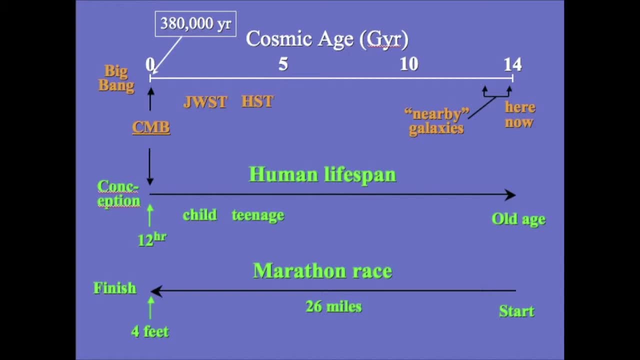 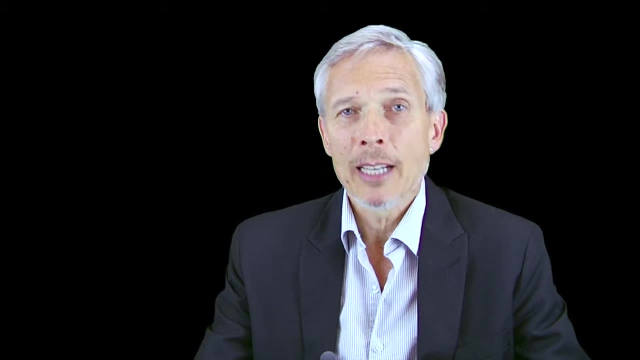 a picture of yourself when you were less than a day old, Or in running a marathon. it's like being just a yard from the beginning of the race. This is an extraordinarily early picture of the universe And it's viewed with extraordinary detail. 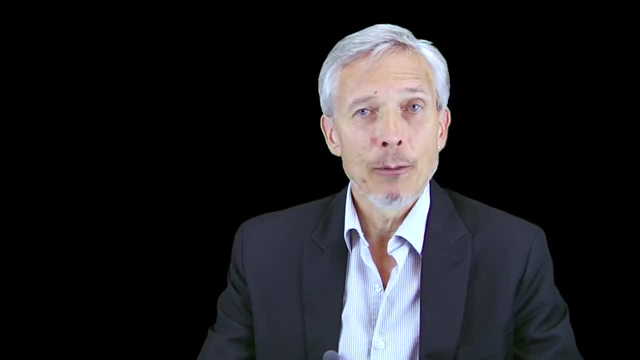 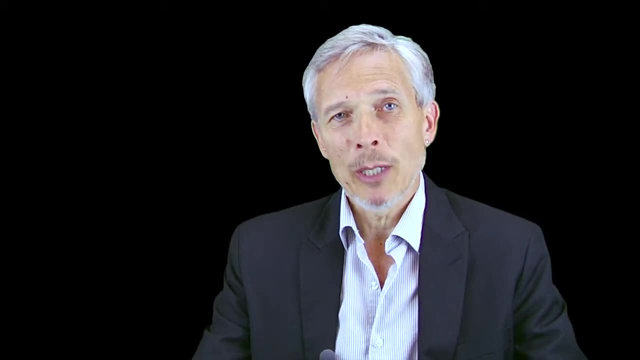 The universe was a very different place when these microwaves were created and released to travel freely through space. The temperature of the universe was 3,000 degrees Kelvin. If anyone had been present to witness this, which of course they weren't, they would have. 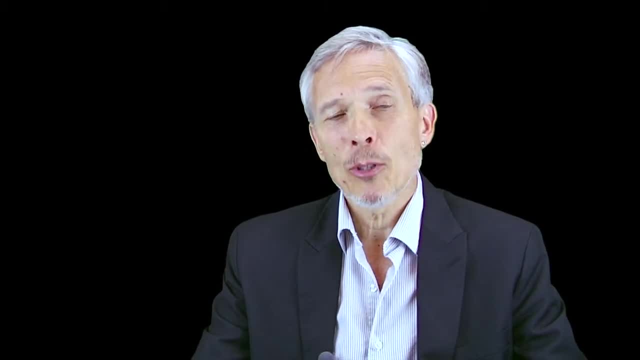 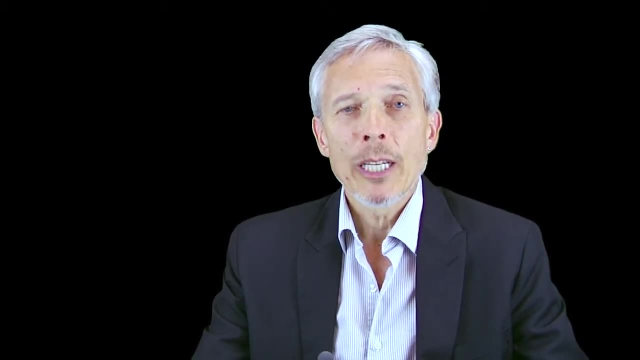 seen a dull red glow. 3,000 degrees is about the temperature of the photosphere of a cool red dwarf And in a sense the microwave background is very analogous to the photosphere of a star. We cannot see into a star because within a region where the planet is we cannot see. 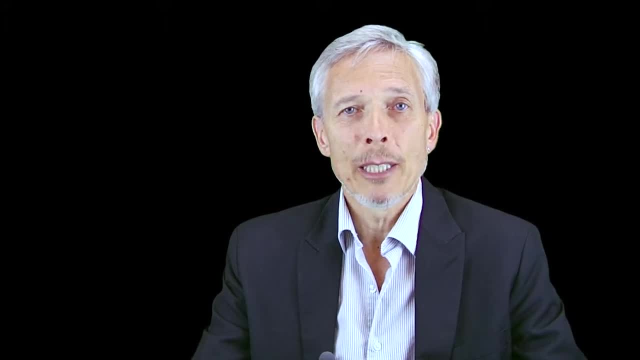 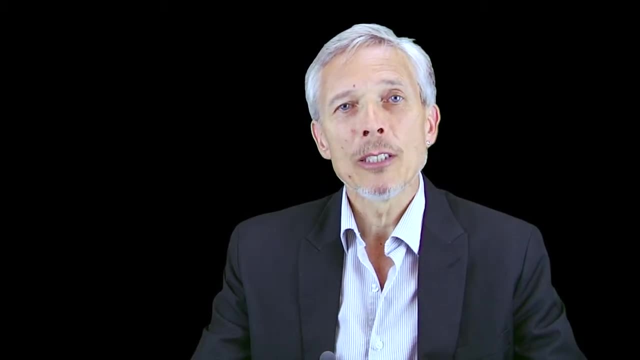 into a region where the plasma density gets high. photons cannot travel freely. The edge of the red dwarf is where the photons start to travel freely. Similarly, with the universe, As it cools, it reaches a density where atoms recombine and radiation can travel freely. 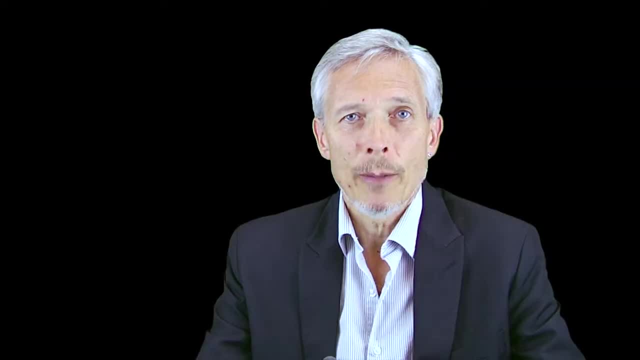 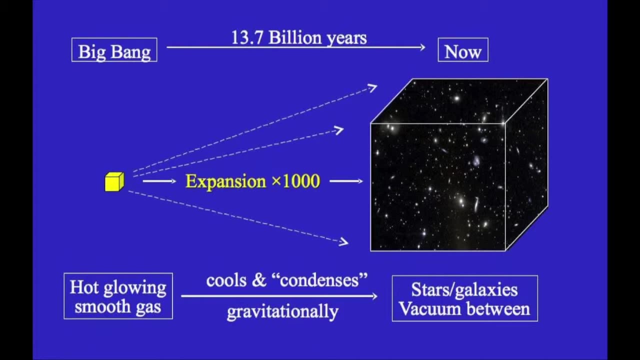 And this corresponded to the time when the universe was as cool as a dwarf star. Since then it has expanded a thousand-fold And by the cosmological redshift those dull red photons, perhaps at the edge of the visible range, have been stretched by a factor of 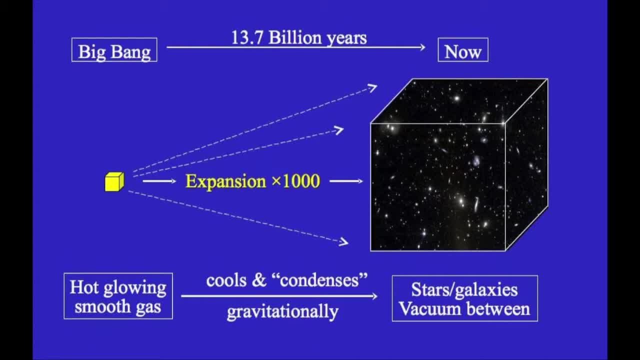 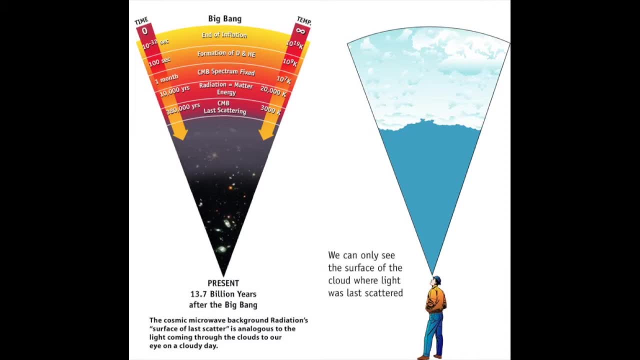 a thousand to be the microwaves we observe with radio telescopes today. So, quite literally, the microwave background corresponds to the visible edge of the universe. Earlier than that, it's a fog that we cannot penetrate with electromagnetic radiation. This is the earliest view we can actually get of the entire universe. Where is the Big? 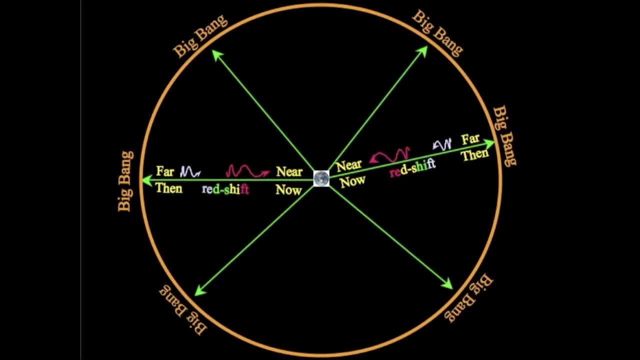 Bang. And where is this microwave radiation? It's everywhere. It fills space: The space between galaxies, spaces within the Milky Way, spaces around the Earth, the room you're sitting in. The Big Bang is all around us because this radiation pervades the universe. The microwave 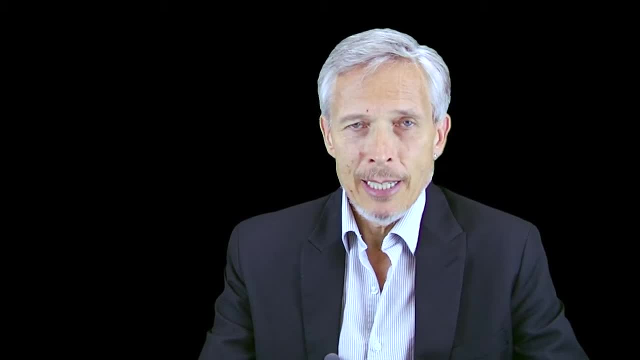 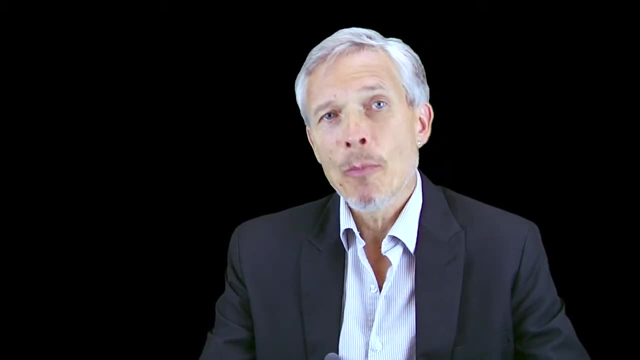 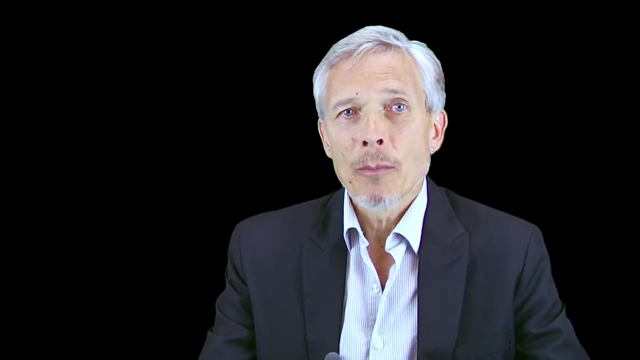 radiation detection was the best evidence clinching the idea that the universe was hotter and denser in the distant past. It's extremely hard to explain this radiation any other way because, remember, there are about a billion of these microwave photons for every atom in the universe. Clever experiments have shown that the microwaves are not local. They do. 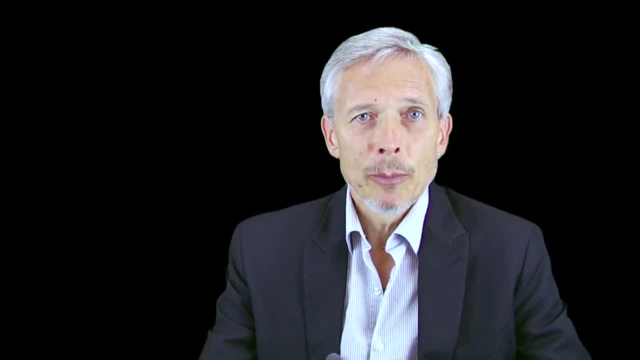 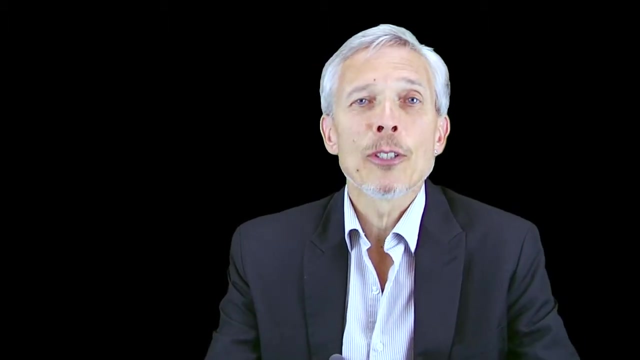 not emerge from our galaxy or the nearby region of the universe, but they are pervasive cosmic source of radiation. There have even been measurements to show indirectly that those microwaves have changed their energy over cosmic time and they have indeed had shorter wavelengths back in the past. Every breath you take contains hundreds of thousands of. 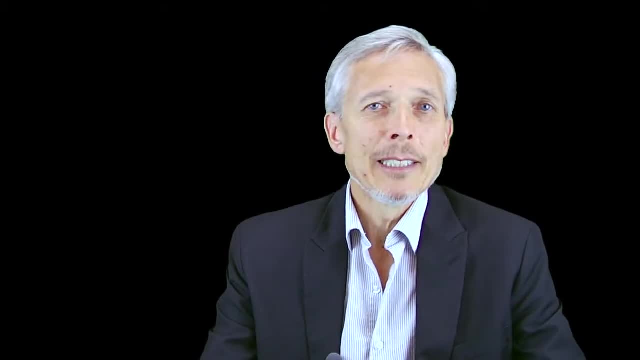 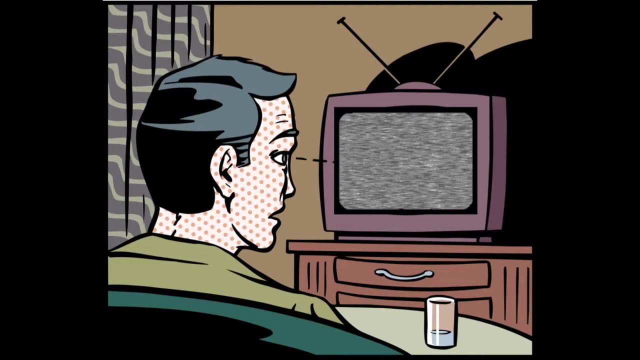 photons from the Big Bang. Most people have plasma or LED TVs now, but if you can find an old-fashioned electron gun or a phosphor tube TV and you tune it between stations, it turns out that about 1% of the speckles correspond to interactions of the phosphor. 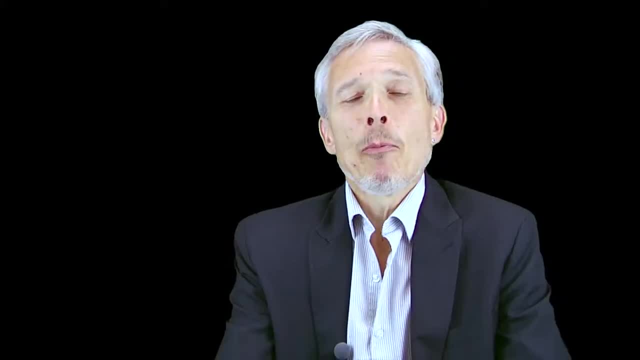 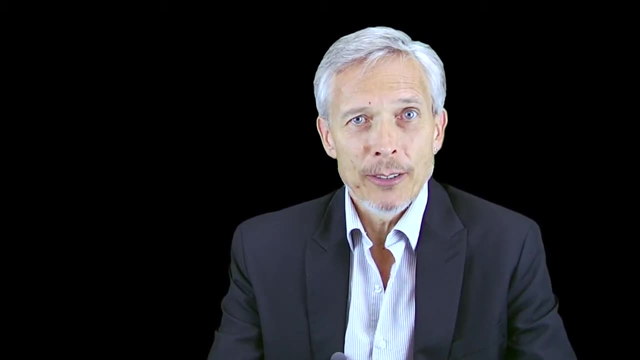 with microwaves from the Big Bang And whatever cable package you might have, I can almost guarantee that watching the Big Bang is more entertaining than most of what you'll find on those hundreds of channels. So some evening just stay in and watch the Big Bang. 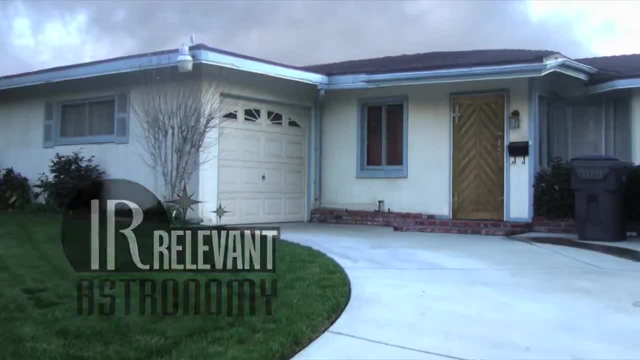 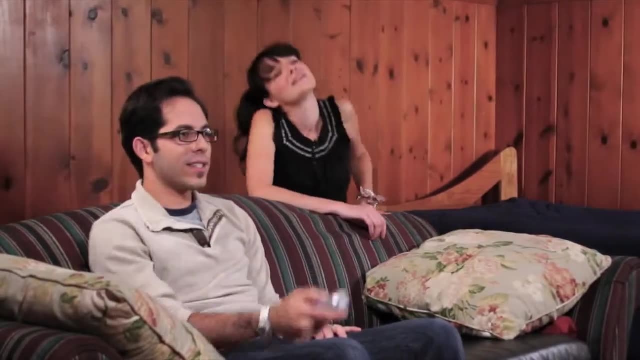 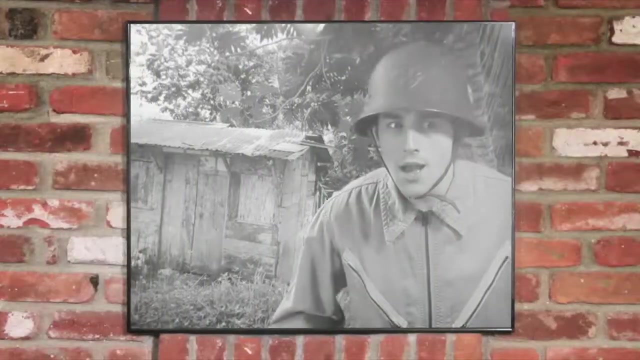 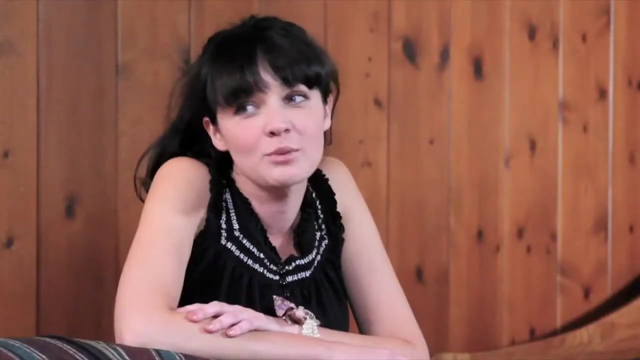 Hey, so what are you in the mood for? Action or action-adventure? Seriously, can we ever watch something without an explosion every five minutes? What? I'm a guy, I like explosions. Aw, cable's out. My digital box is loose. You have to jiggle it, Or we could just watch the Big Bang. 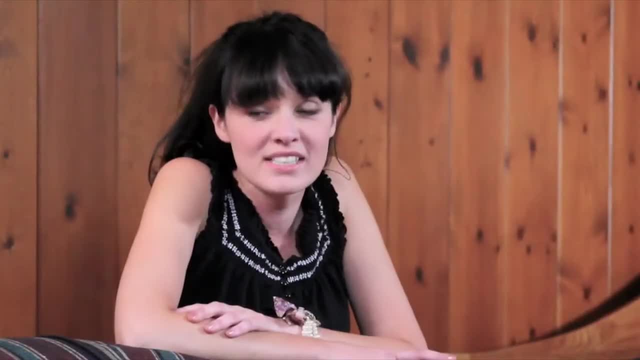 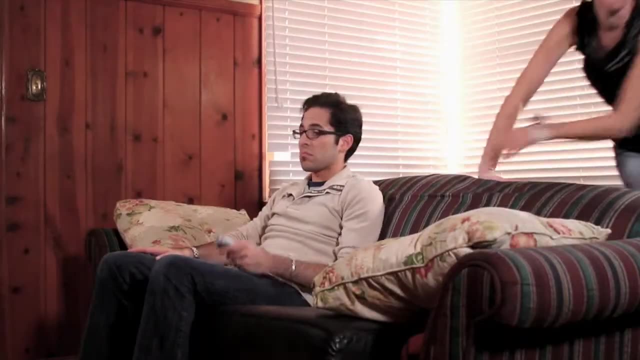 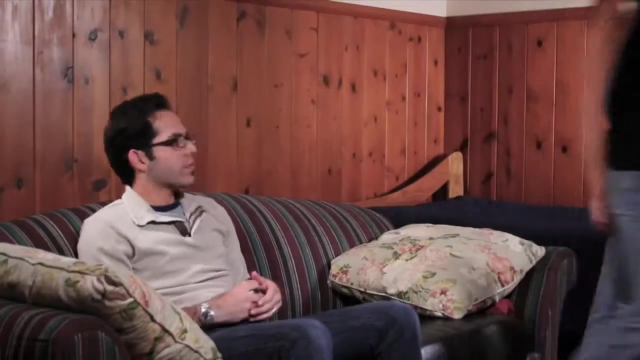 Yeah, Wait what? The Big Bang. Whenever you see static on an analog TV like this, a small part of that static is actually residual radiation from the Big Bang. I can watch that. We are not watching static. Find something else. 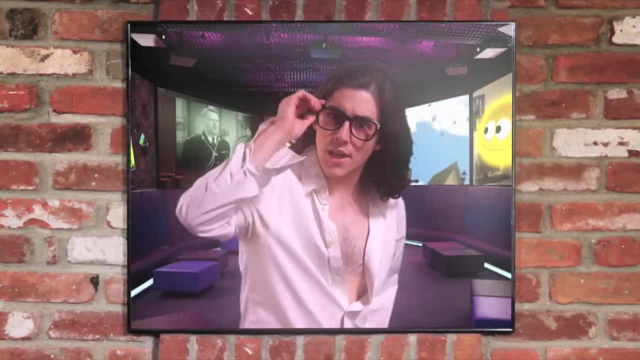 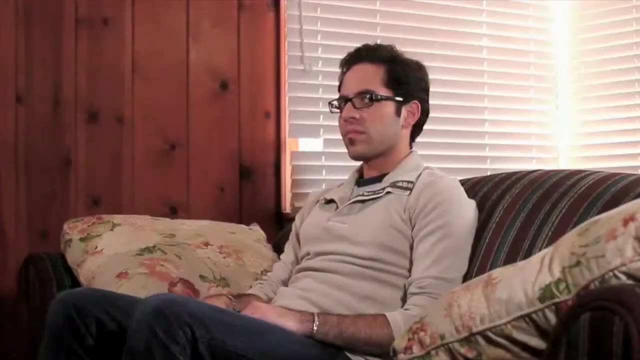 I'm flipping channels on my TV set. Haven't found something worth watching yet. Suddenly the fuzz is setting in. It's good, old-fashioned entertainment. It's been proven to be true that some percent of static is fogging you. It's radiation that we can't see from the Big Bang. 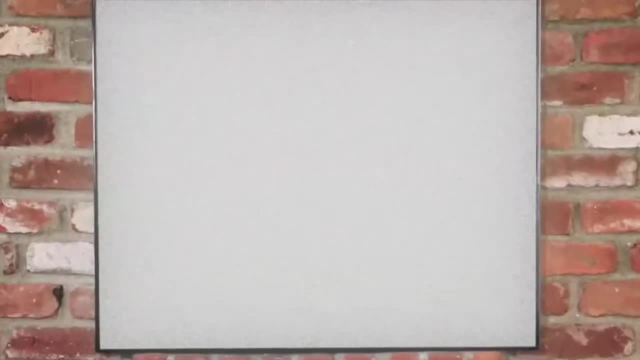 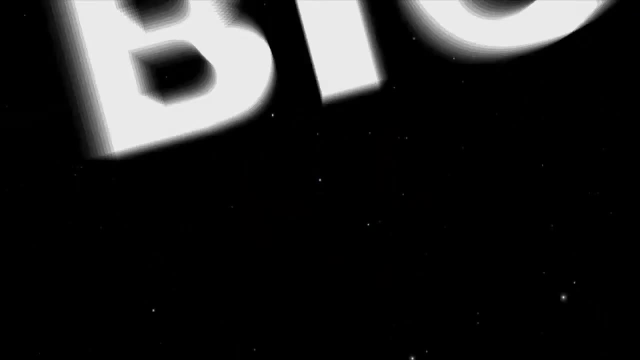 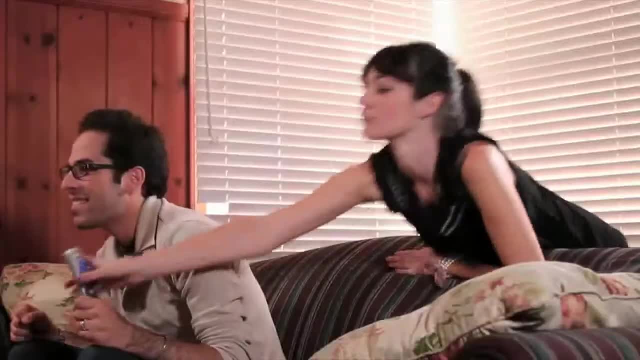 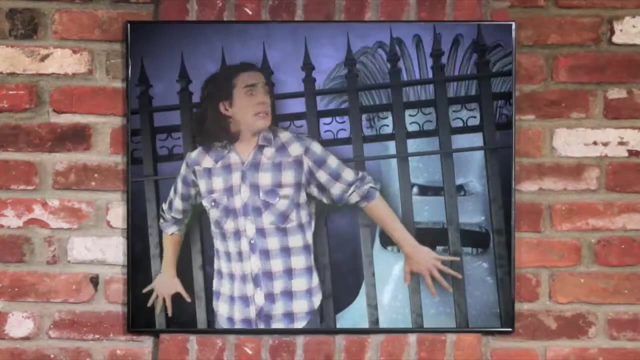 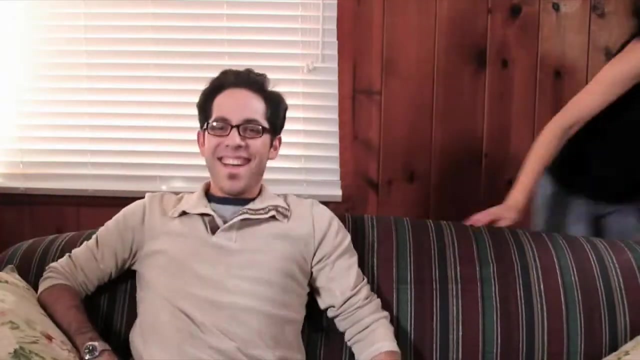 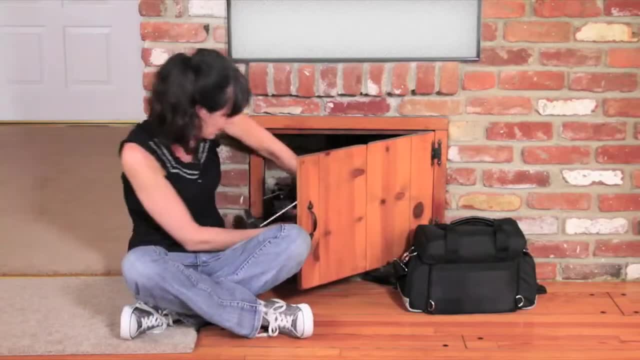 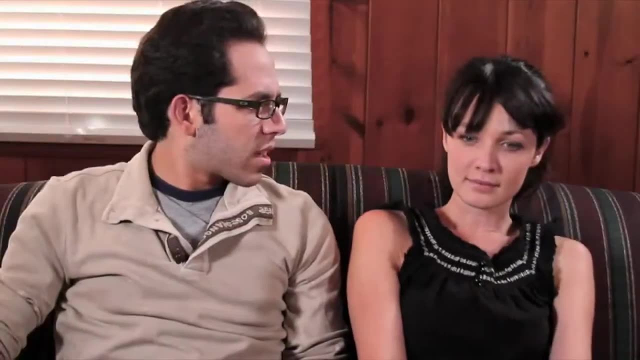 We should study this. That's why the European Space Agency, with help from NASA, created the Planck Space Observatory to help study this cosmic microwave background. What's Planck? I'm glad you asked. Planck found a way to see that light. 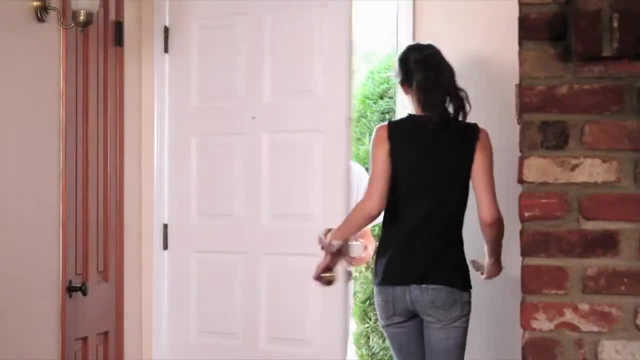 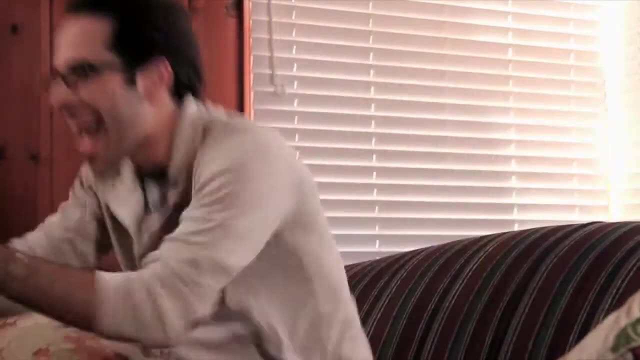 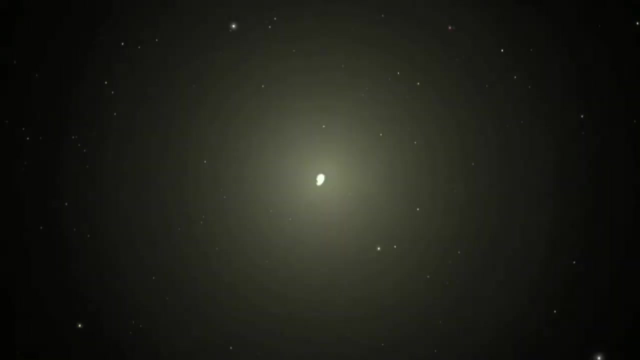 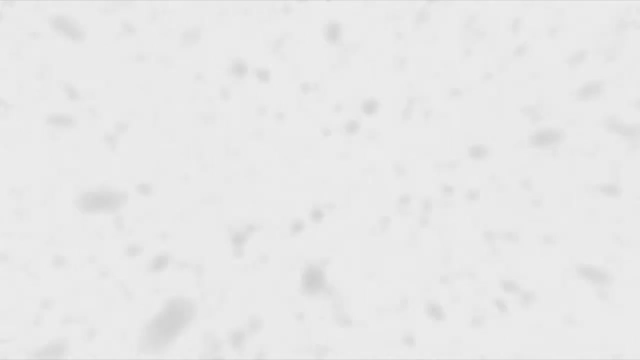 Subtracting dust from the pictures of the sky at night. A microwave- that's worth what it was, And I can see it in my TV voice. It's been proven to be true That some sort of static is forming you. It's radiation that we can see From the big bang. big bang, big bang on your TV. 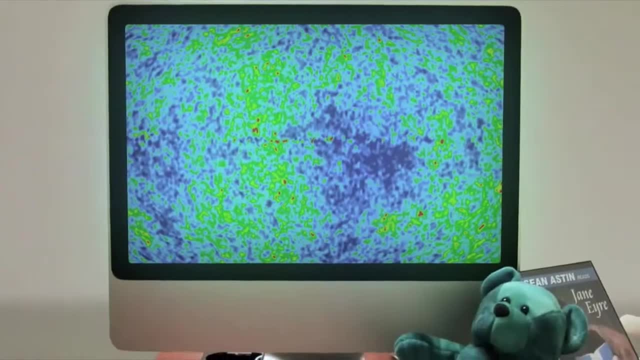 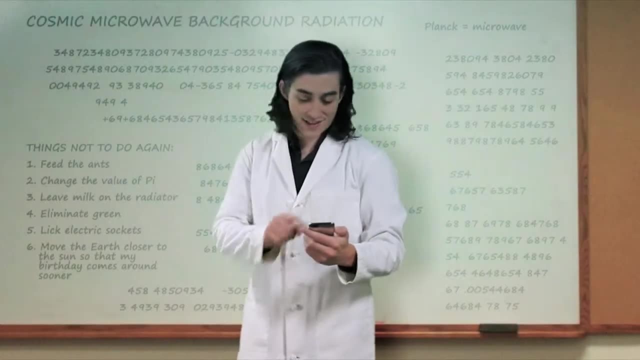 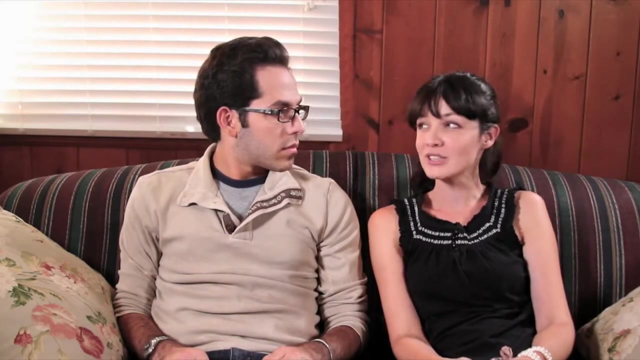 And by scanning the sky and dissecting what they found, Cosmologists believe they know the shape of space around. The static mathematics have been translated to this sound. This sound was converted from data of big bang radiation by a university professor in Seattle. Yeah, I can feel it. 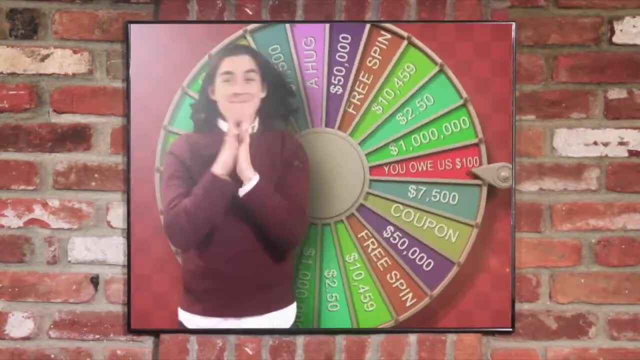 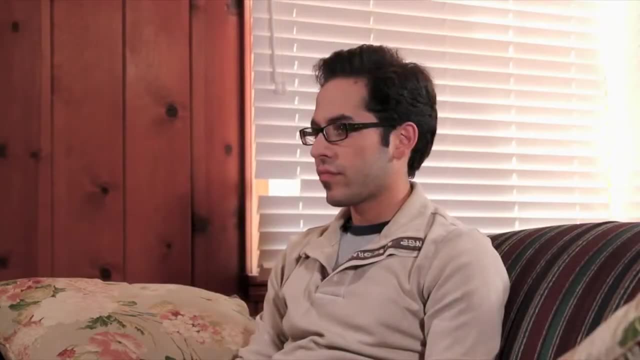 With hundreds of channels on cable and broadband. I'd rather sit at home and watch the universe expand. If inflation had a station, it would be my destination, But for now I'm going to stay here And the flicker of existence on the clicker in my hand. 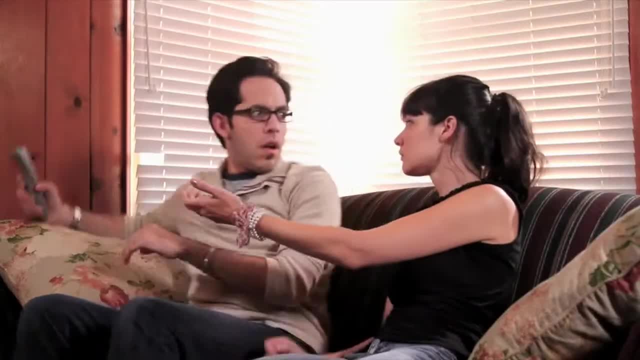 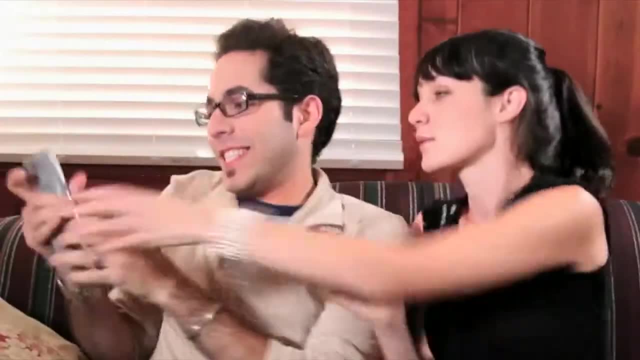 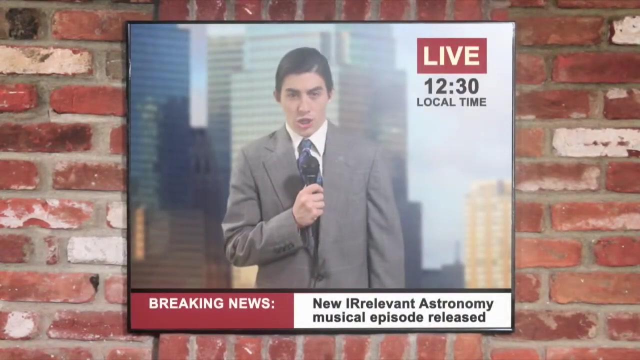 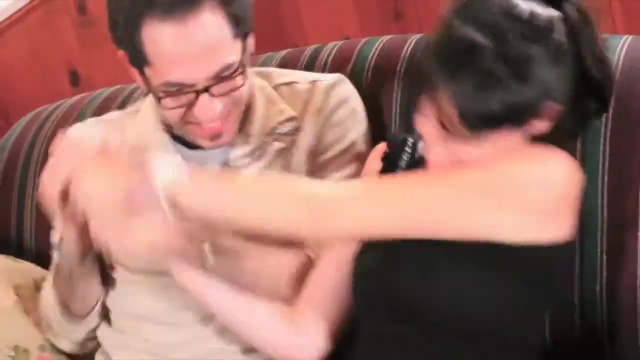 OK, that's it, Give me the remote. No, It's been proven to be true That some sort of static is forming you. It's radiation that we can see From the big bang, big bang, big bang on your TV. And by scanning the sky and dissecting what they found, 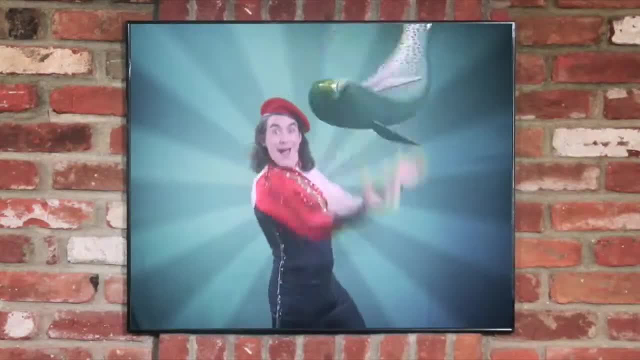 Cosmologists believe they know the shape of space around And by scanning the sky and dissecting what they found, It's the moment you can see. It's the moment you can see. It's the moment you can see The Big Bang, Big Bang, Big Bang on your TV. 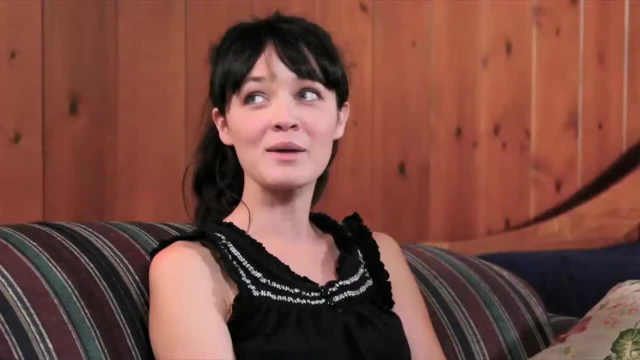 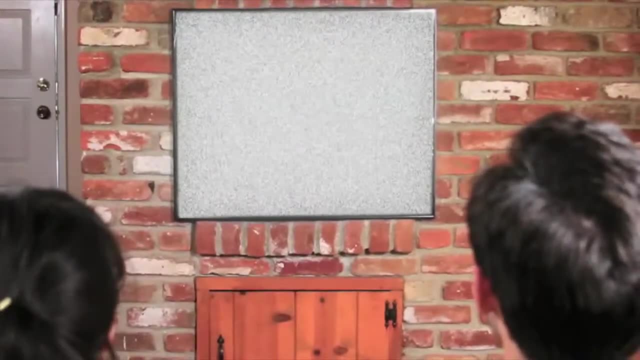 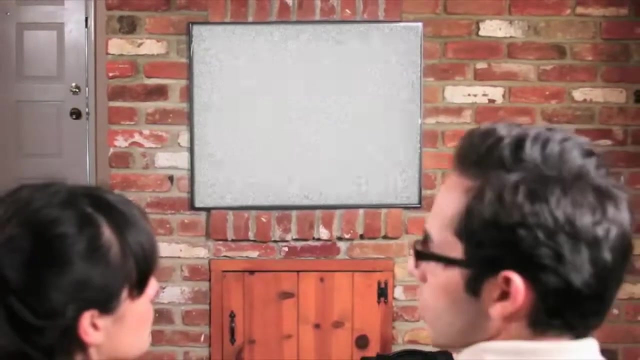 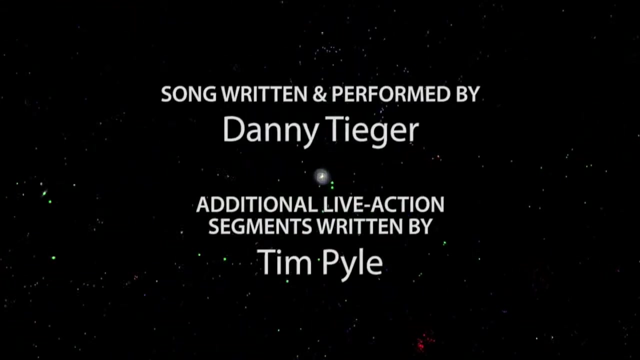 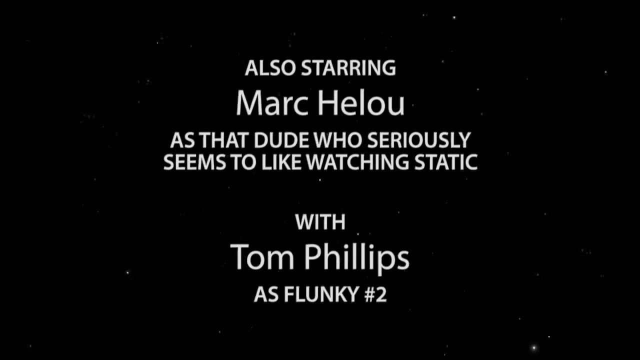 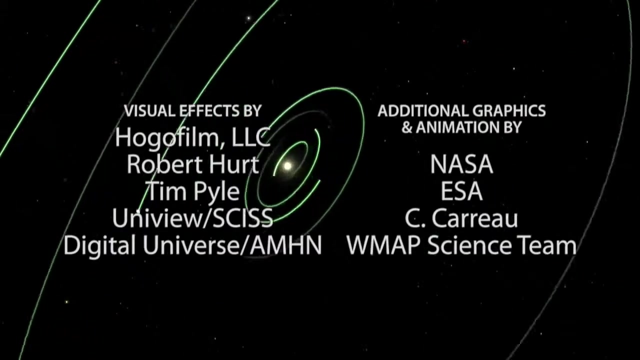 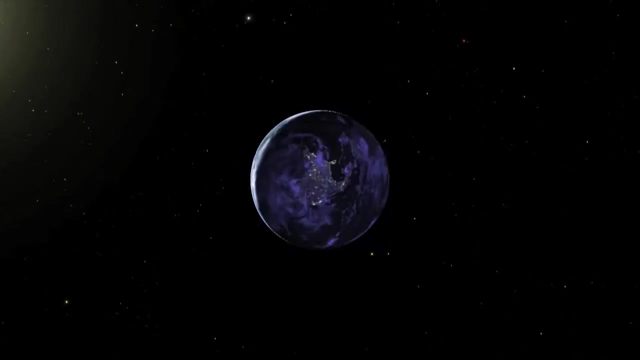 Haha, I win. Fine, we can watch The Big Bang, but tomorrow I choose the show. You know, I think this one's a repeat. You know, I think this one's a repeat. Big Bang, Big Bang on your TV. 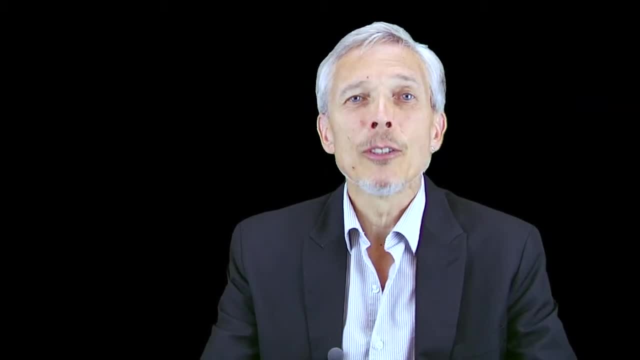 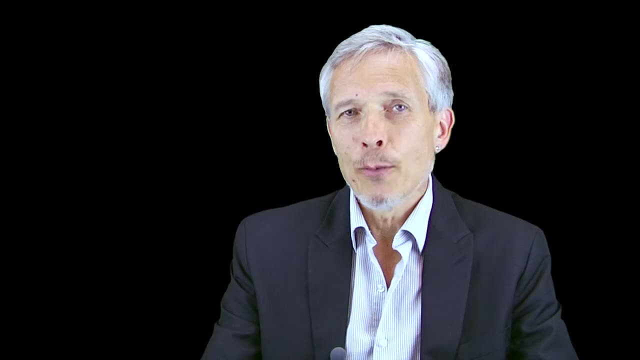 Mark Whittle at the University of Virginia has even managed to sonify The Big Bang, or turn the astrophysics of the early universe into a sound analog. What you will hear is the first 10 million years of the universe, compressed in time to about 10 seconds. 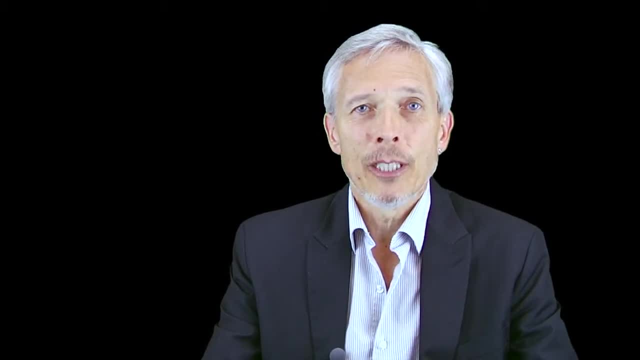 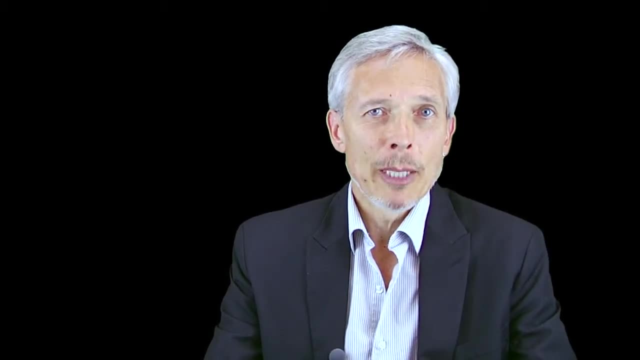 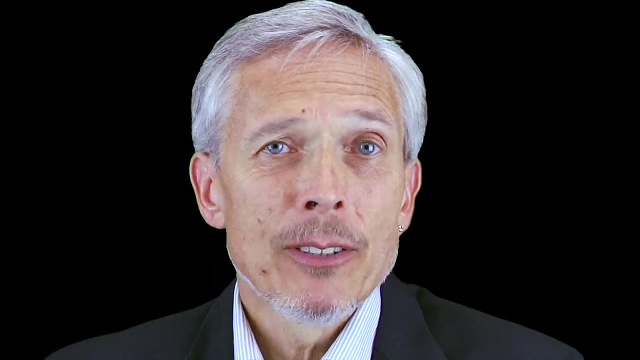 and taken up in frequency by 54 octaves into the audible range, Because most of these vibrations in the plasma were extremely low frequency. This is the sound of The Big Bang, The most dramatic evidence that the universe had an early hot dense phase. 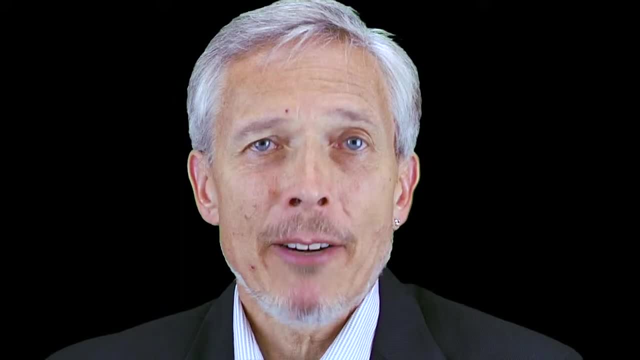 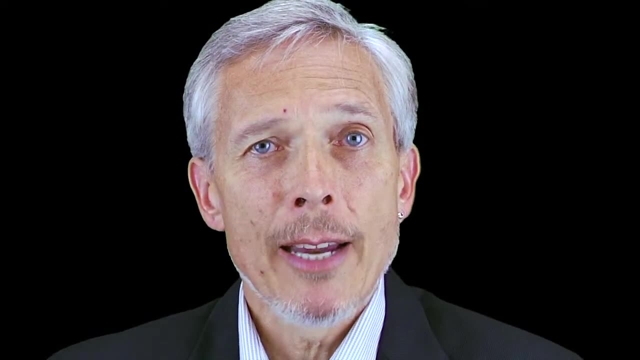 and that The Big Bang actually occurred is the microwave background radiation Discovered in 1965, it's an almost uniform signal of microwaves in every direction of the sky, representing radiation released into the spaces between galaxies- the heat bath from the early hot Big Bang.